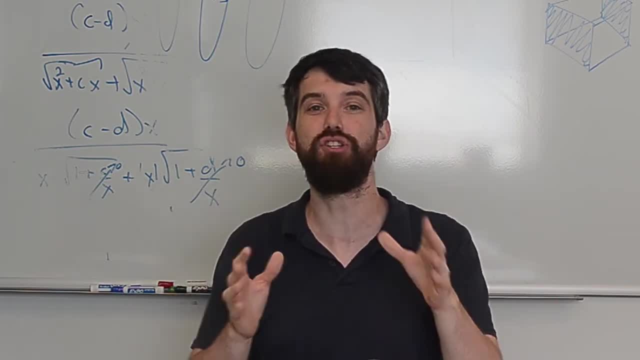 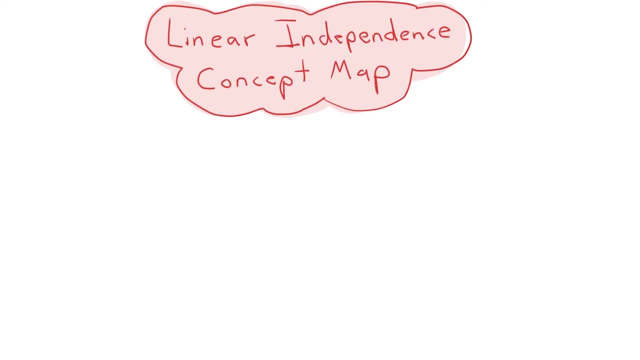 So in this video I'm going to go and sort of pretend to be a student and I'm going to show you how I would make a concept map. My concept map is going to be about linear independence. Before I do anything else, I want to write down what is the definition and I've sort of forgotten. so let me go look it up. 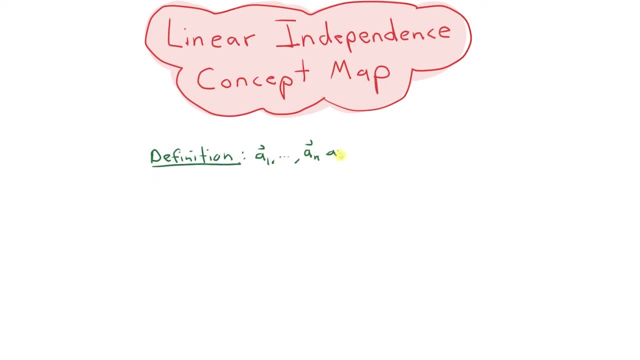 Okay, so the definition is a list of vectors: a1 to d1.. They are literally independent. if and then. apparently the condition is: x1, a1 plus all the way down to xn. a n is equal to 0 implies x1 is equal to blah, blah, blah equals xn is equal to 0. 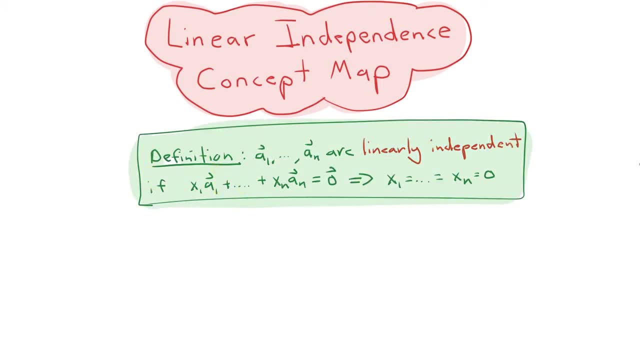 All right. so what on earth does that mean? How do I even start to piece this apart? Well, I think the first thing I'm going to do is just sort of figure out what things are, what x1 down to xn. those don't have vector hats on them, and so they're going to be scalars. 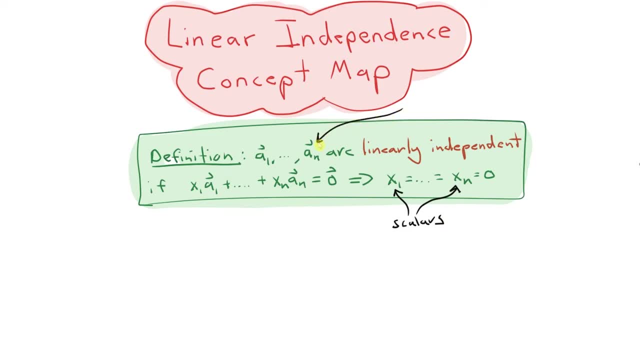 The a's. those are vectors that got little vector hats. So I think that the a1 down to the a n, those are something living in Rn. Now what else do I know about this? Okay, I see that this x1, a1 plus all the way down to xn a n- I've seen that before. 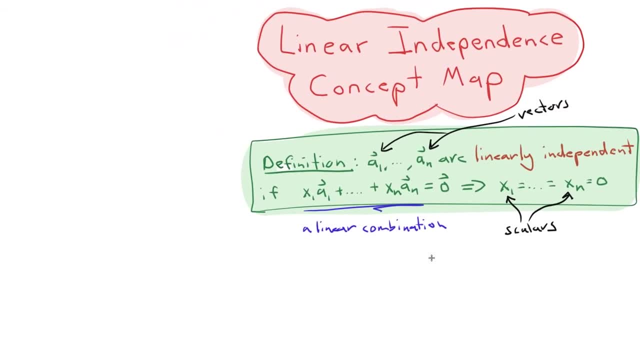 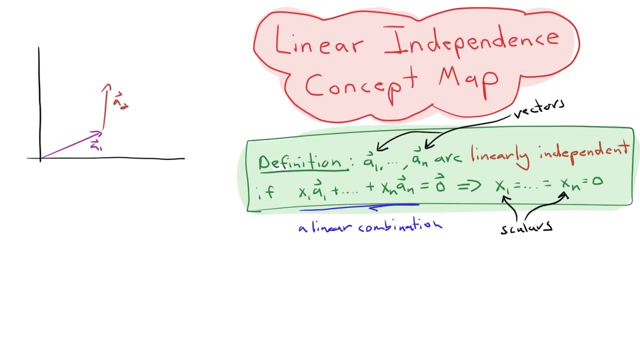 That's a linear combination, So let me go and try to sketch that out. Okay, I'm going to draw two different vectors, an a1 and an a2, and there's no way I can get around to 0. There's no way I can take a linear combination of those getting to 0 unless unless I make the length of the a1 and the length of the a2 0 by multiplying. 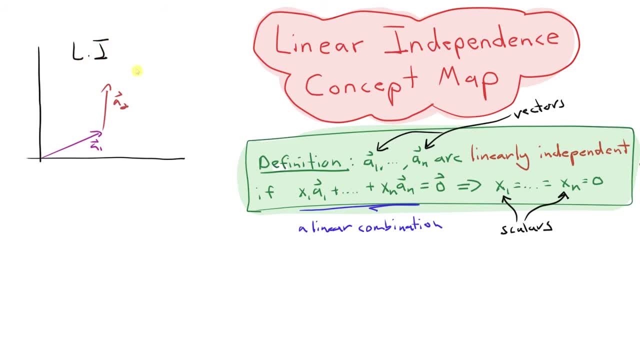 by scalars that are 0. So this scenario I'm going to say is linearly independent, that I cannot add to 0.. Okay, what about the other scenario? If I create an axis, then I'm trying to imagine some linear combination that adds up to 0. 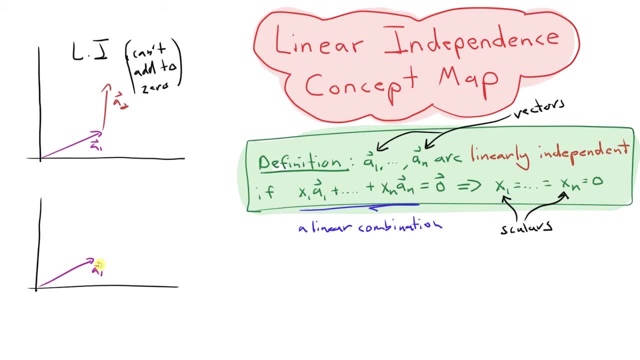 Well, maybe it looks like this: Maybe I've got an a1, and I've got an a2, and then I've got an a3, and if I go around that loop I get back down to 0.. So that's the linear combination, that's equal to 0. 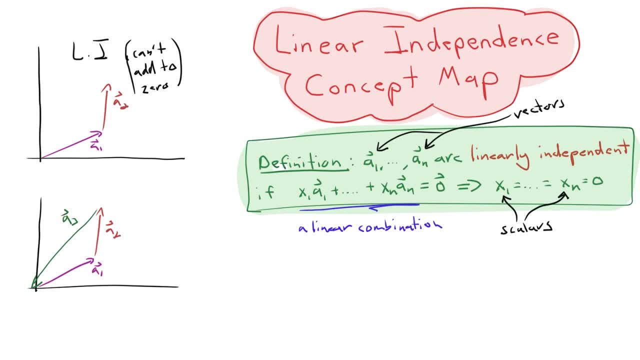 There's a1, a2, a3 that I've sketched and I see that indeed it adds to 0. But then if I look at the scalars here, these vectors all have lengths, so the the scales are not 0.. 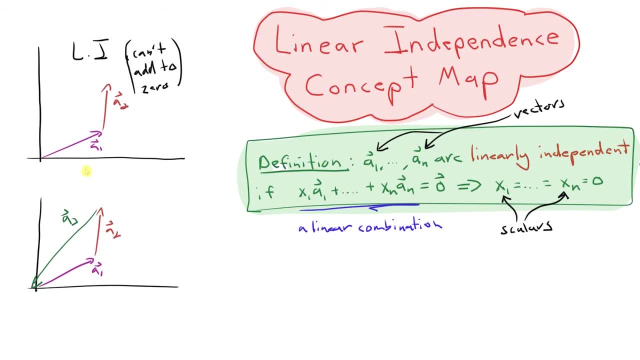 So, indeed, by this definition, that this situation where I can kind of make a triangle, that that is going to be a linearly dependent one where they all add to 0. Okay, so that's sort of how I visualize it. linearly independent says there's no linear dependencies. 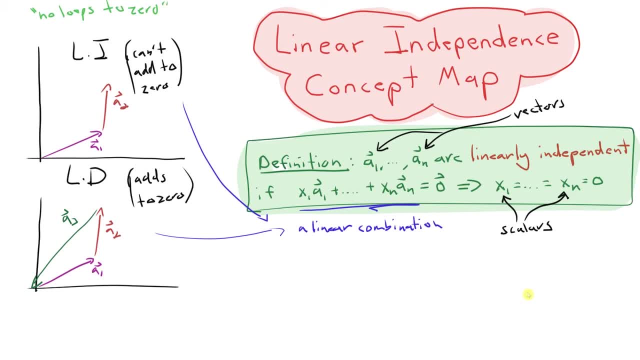 There's none of these loops to 0.. Now, what else can I do? Well, okay, the x1, a1 all the way down to xn, an. that's a linear combination. before a different context I've seen linear combinations in is the definition of the matrix. 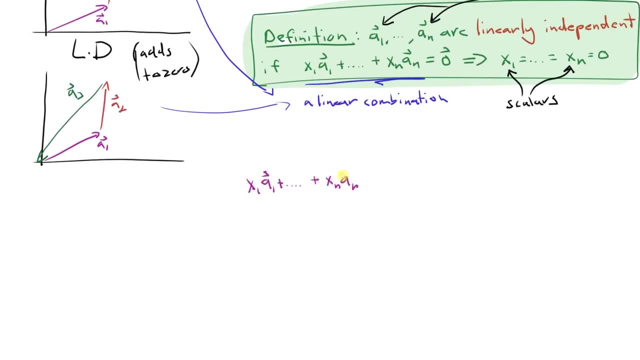 Vector product, So I can come and write that out, that this is just going to equal to a times x, where a is just going to be some matrix that has the columns a1 down to an. Now the linear combination might be replaced by ax. 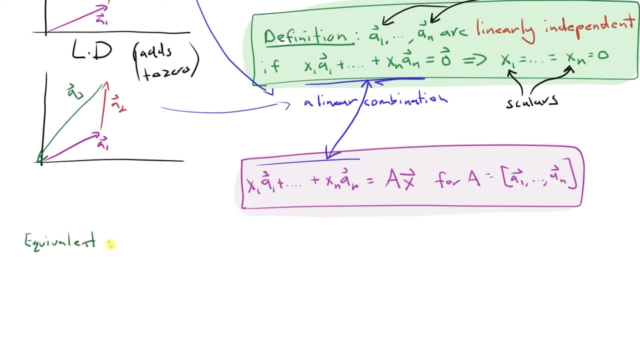 but it's really up on the original definition is ax equal to 0. So really saying literally independent means that if you have ax equal to 0, then you only have x equal to 0 as a solution. In fact, x equal to 0 is always a solution. 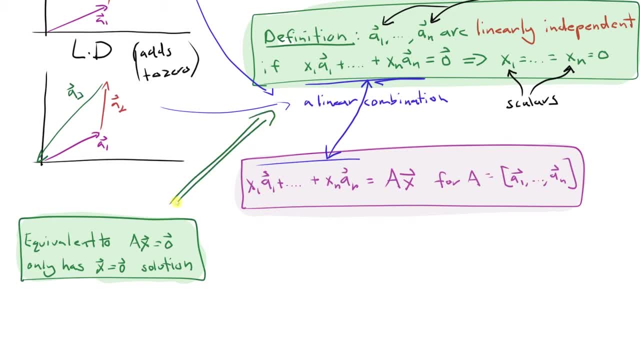 We're really saying we're learning that what makes ax equal to 0 independent is that there's not some other solution. This means this is a homogeneous system. Ax equal to 0 is homogeneous. Okay, let's do an example of this. 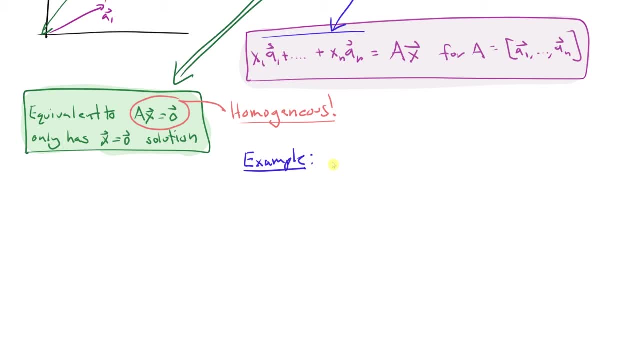 Let's try to put that on our concept map So we sort of know how to connect these ideas. A concrete example it's always nice to have. How about one where I give you three different vectors: 1, 2, 1, 2, 0, 1, and minus 1, 1.. 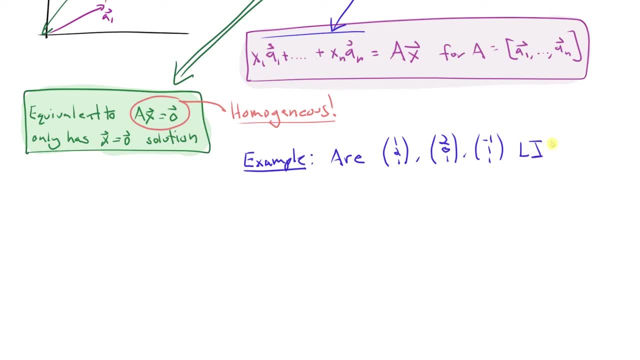 And the question might read: is it linearly independent? Is it linearly independent? I don't know. So what's my process? Well, what we had just seen was that I need to go and solve ax equal to 0. So why don't I go and try to put that system here? 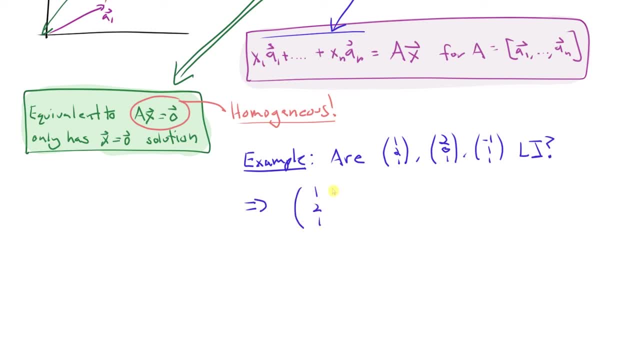 I'm going to write down a homogeneous system. So then I'm going to put my matrix: 1, 2, 1, 2, 0, 1, minus 1, 1, 1.. I'm going to append the 0 vector because it's the homogeneous. 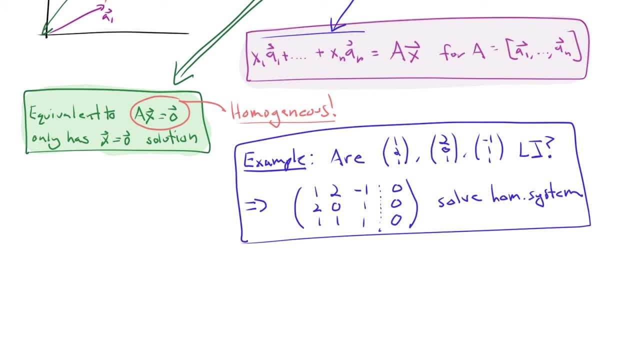 and then I just need to solve that. It's a question of whether there's going to be just a 0 solution, whether, in fact, there's going to be more, All right. so how do I actually do this? Well, okay, I think this technique would go to do row reductions. 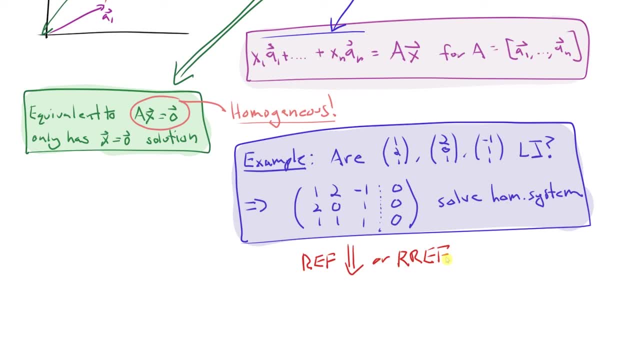 put into REF or RREF. And when we go into RREF or RREF, there's actually two possibilities: Either one solution or infinitely many solutions. You might, by the way, think: well, hold on, is it possible that you had 0 solutions? 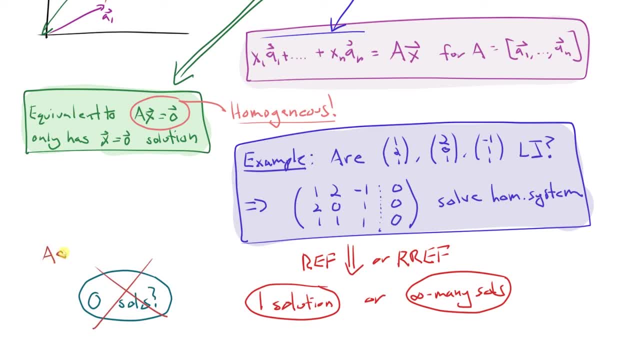 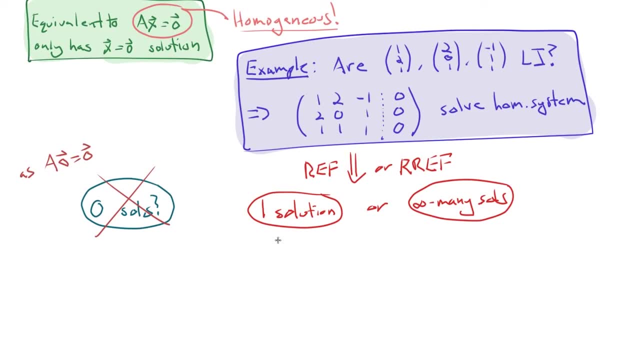 Well, no, that's not one of the possibilities, because a times 0 is always equal to 0, so 0 solutions isn't a possibility. They've got 1 or infinitely many. Now, having one solution meant that there were no free columns. 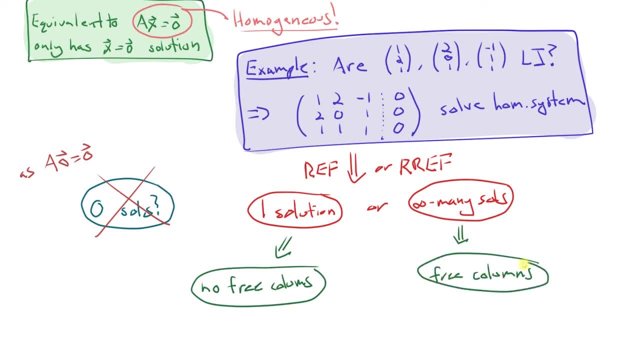 Well, having infinitely many solutions meant there was a free column, So that's another way I can go and analyze what linearly independence is. It has something to do with, when you put the matrix in RREF or just REF, whether it's got one solution or infinitely many. 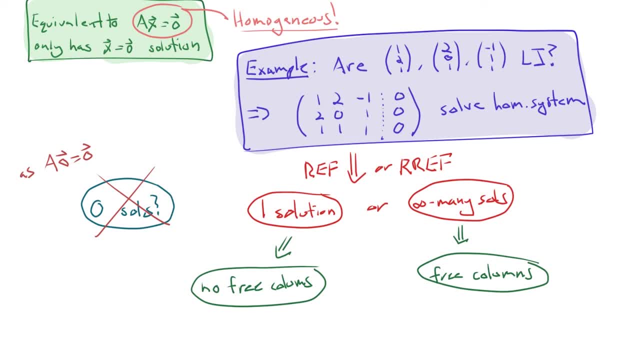 which is just the same thing as saying: does it have no free columns or does it have free columns, Okay? well, I can go a whole step further. If there's no free columns, that means every single column has a leading 1 in it. 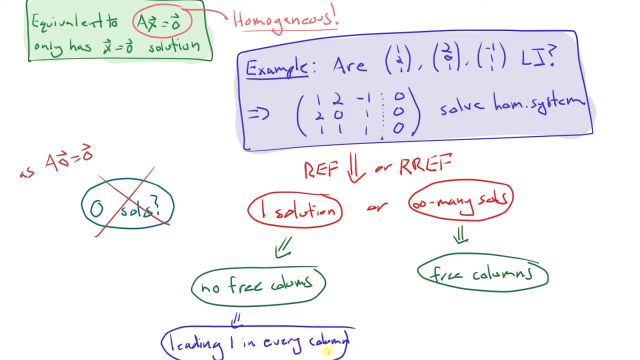 A free column is one without a leading 1.. So these ones on the left here, where there's the one solution, the no free columns, the leading 1 in every column. this is the scenario where it's linearly independent, that you've got your linear combination equal to 0. 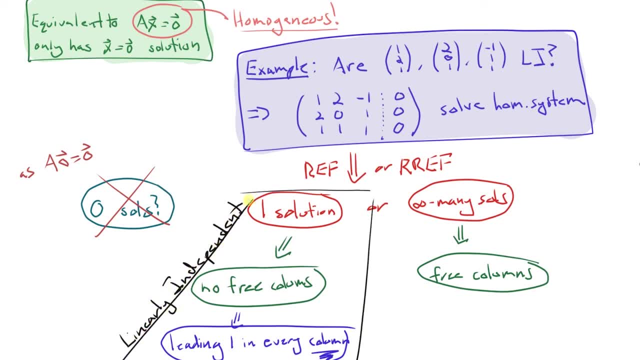 and you only have the coefficients all being 0 allowed. That's linearly independent. And then the other side, where you're talking about infinitely many solutions with a free column, a column with no leading 1, that is going to be linearly dependent. 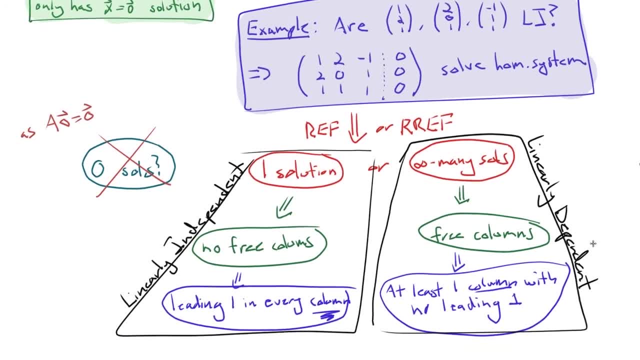 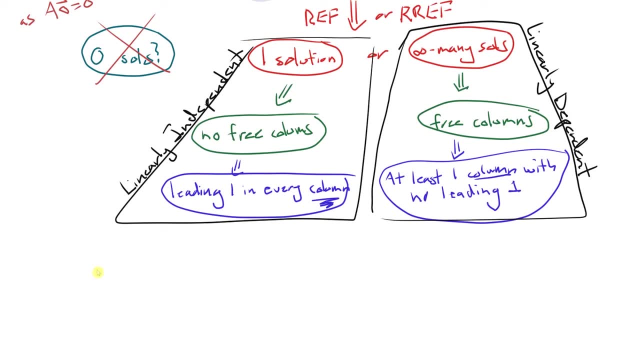 One more thing I might want to add to this is the idea of 1 to 1.. That was another concept that was sort of brought up. Is that related? Well, 1 to 1 meant that the transformation that took the vector x and took it to Ax. 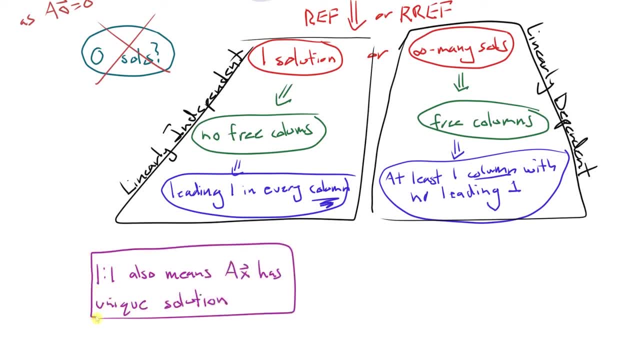 that had a unique solution. That's what it meant to be 1 to 1.. It meant that Ax had a unique solution. By the way, all these different implications are actually double implications. They work both ways, as in no free columns. 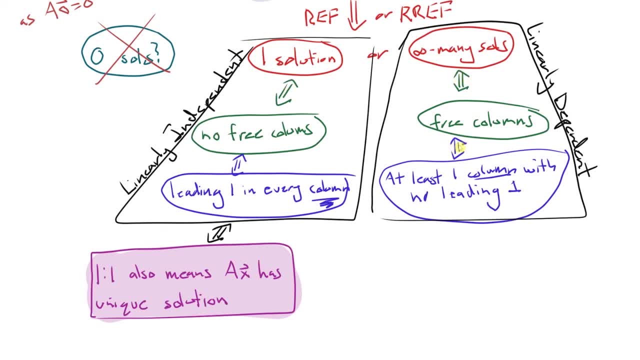 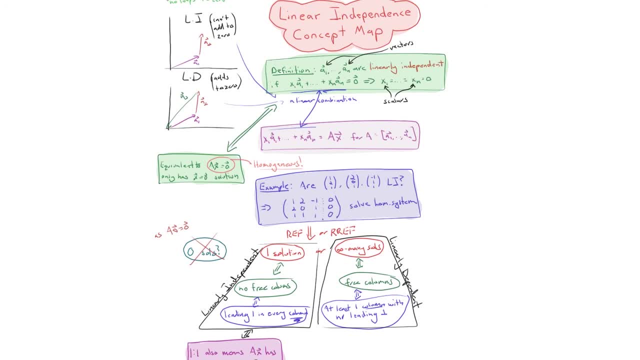 if, and only if, one solution. All right, Zooming out, we can see the entire concept map that I've created, And indeed I can add quite a bit more to this. And as we go on in the course, we're going to see topic after topic after topic.